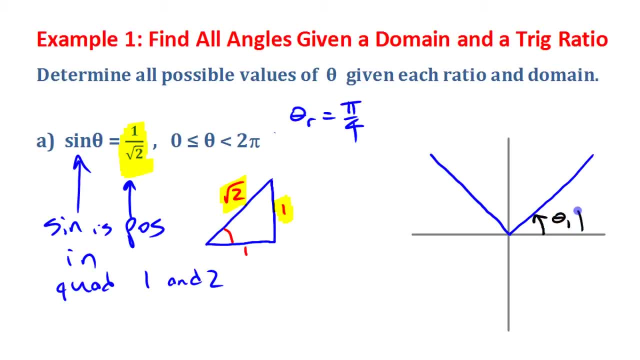 I'm going to call it theta one, And one is over to here. I'm going to call it theta two, And then we can pretty much write what those are right away. right, If these were the reference angles in here. Theta one is the reference angle pi over four. 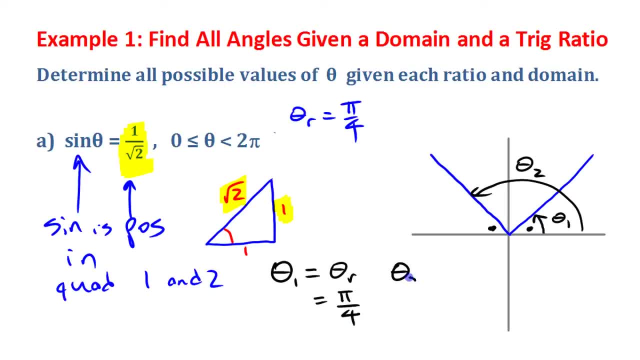 And theta two. theta two is pi minus that reference angle, three pi over four. So there's actually two angles. There's actually two angles that meet this criteria, As in there's two angles that have a sine of one over root, two within one full turn here, right? 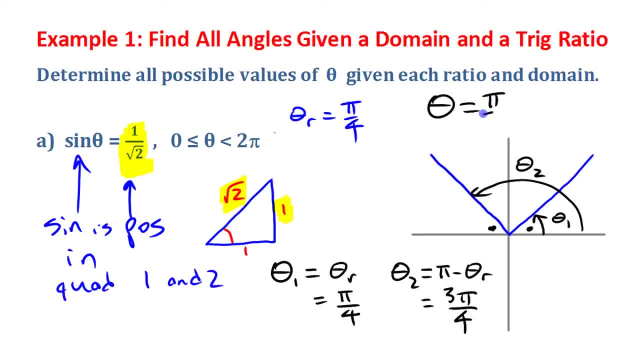 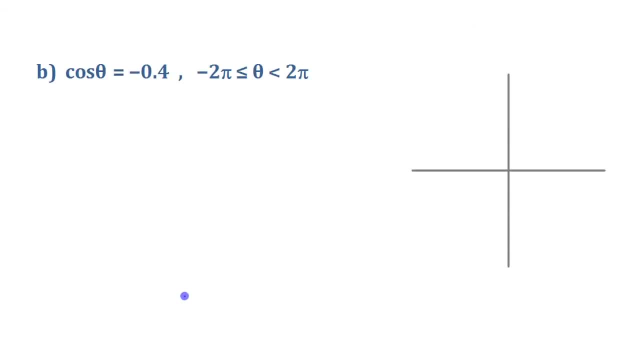 So we can just put up at the top here. Theta could be pi over four or three pi over four. all right, Now let's look at the second one. So this time we're looking for where cosine is negative 0.4.. 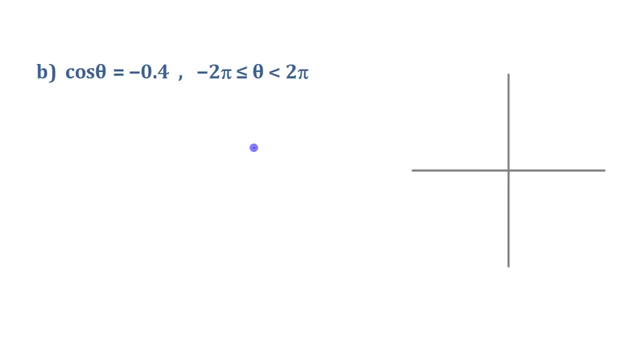 And we're looking in a bigger domain here, because we're looking all the way from one clockwise rotation All the way to one counterclockwise rotation. Now, this 0.4 here is not a special ratio out of one of those special triangles. 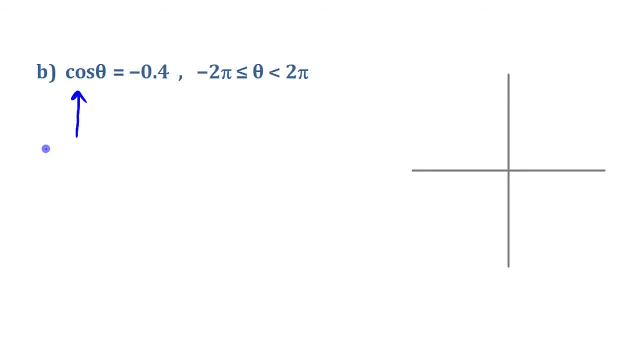 So we're going to have to use our calculator for this. First thing we should look at here is: cosine is a negative number, And think about where our angles are going to be. Cosine is negative in quadrants two and three. We're going to be looking at quadrant two and three. 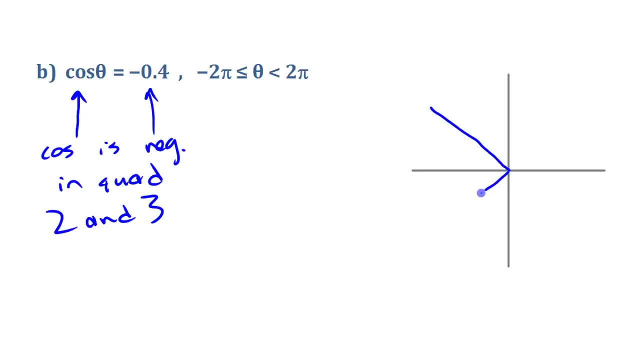 I'm just going to roughly draw two angles in here. They might not be kind of to say The scale or anything like that, but it'll at least let us think about what we're looking at here. We need to find our reference angle. to find the reference angle, 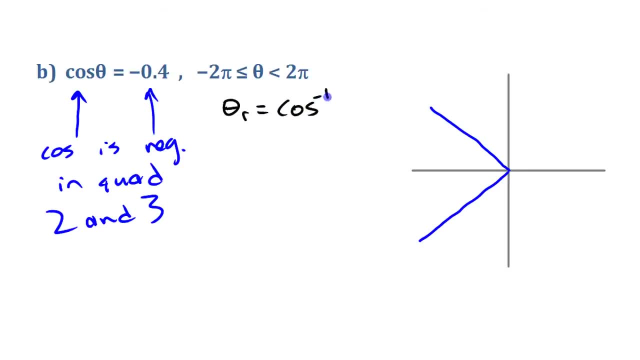 What we're going to do is we're going to use our calculator and say cosine inverse of positive 0.4.. Notice that I don't put the negative in here. It says cosines negative 0.4, but I'm only putting 0.4 in here because it's a lot easier to put the, to not put the negative in, so that we know we get a positive acute angle less than 90, less than pi over two. 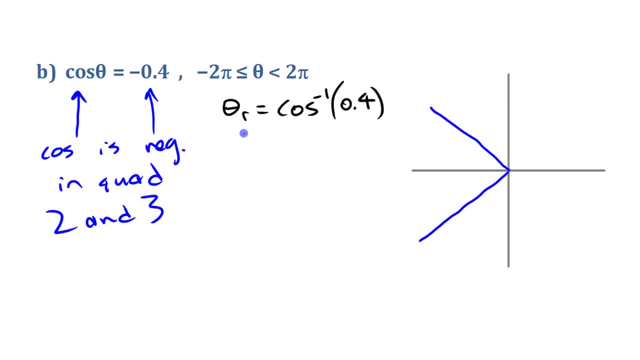 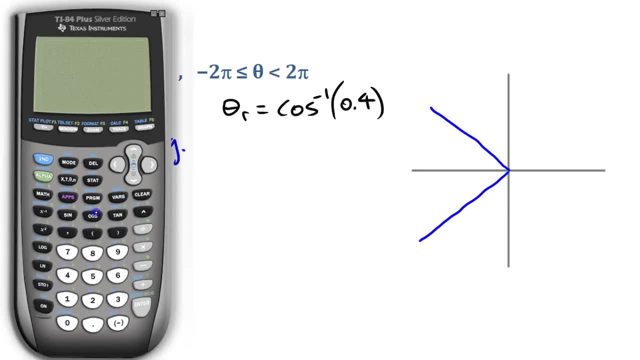 And then Work with that in each of the other quadrants. So get our calculator out here and make sure it's in radian mode, which it is, And we're going to go cosine inverse of 0.4- 1.16.. 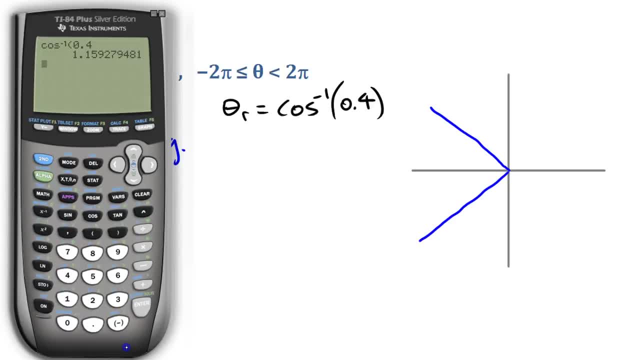 If we're going to two decimal places. I am going to store that number, though on my calculator you can store it as anything. I'm going to store it as X, just because that's easy to get to. Then I can use that again here. 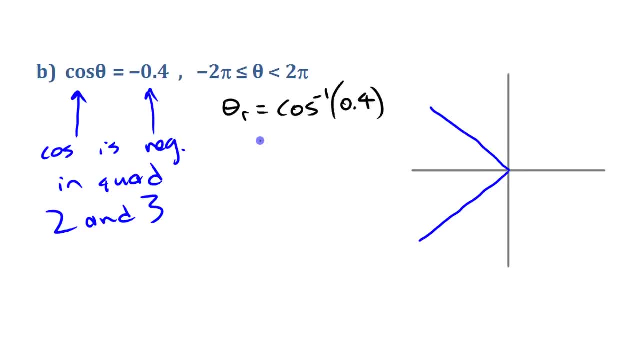 All right. So first of all, I'm just going to put down roughly that that's 1.16 for theater reference, And then I'm going to think about what the angles I'm looking for. One of the angles I'm looking for is right there. 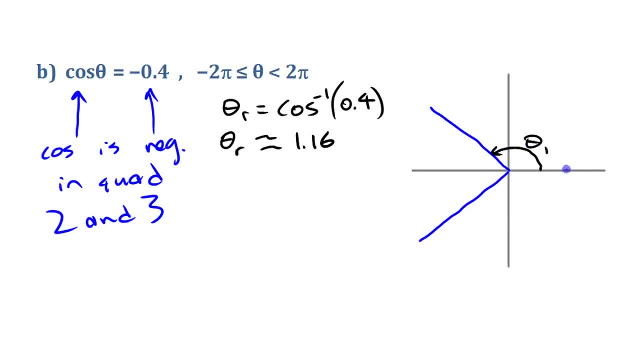 I'm going to call that Theta one. Another angle I'm looking for is: right, here, I'm going to call that Theta two. And then we're also going to be looking for angles that are the other direction as well. Right, We're also looking for this angle. 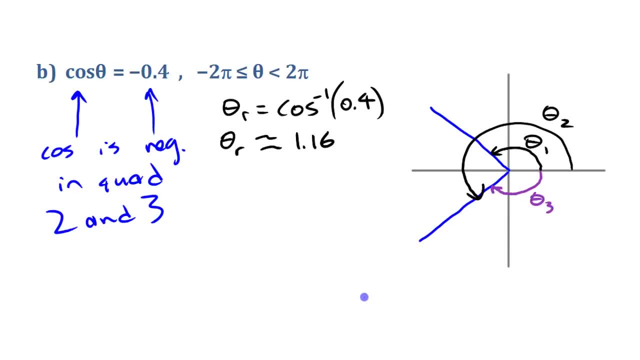 I'm going to call that Theta three. Theta three and Theta one here are going to be just opposites of each other, though, So there's not really more to find, And then the same goes for this. That's just going to be the opposite. 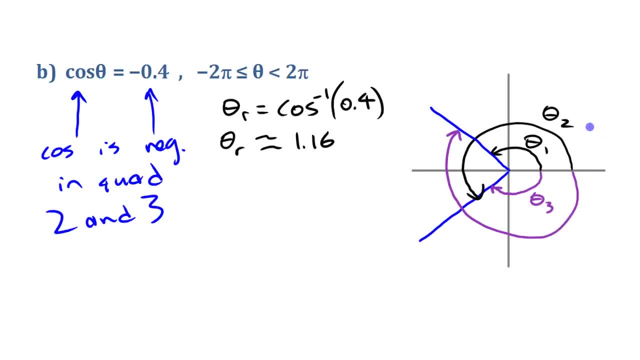 It's going to be the negative of this, All right. So we really have two numerical values to find and then we can write all four angles. I erased my Theta four there. Other than that, we're going to be outside of our domain, that we're given. 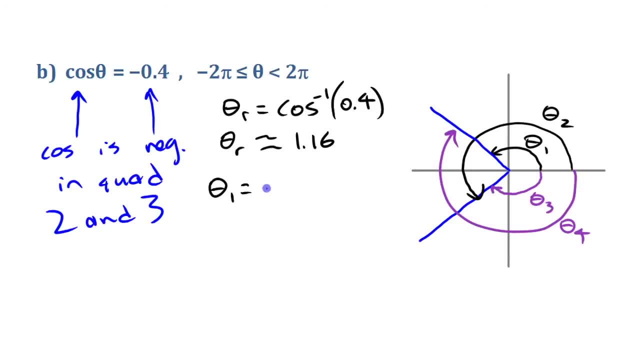 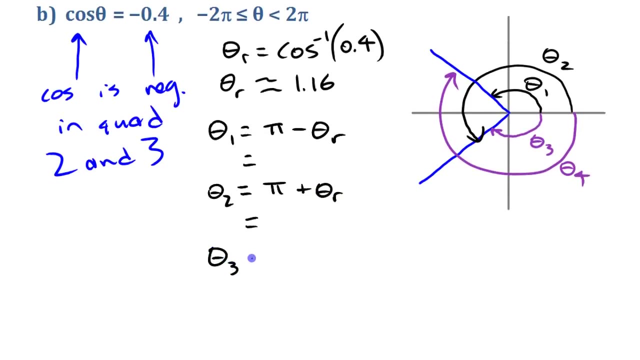 Okay, So we're going to have: Theta one is Pi minus Theta reference and Theta two is going to be Pi plus Theta reference, Quadrant three. Theta three is going to be negative. Theta one and Theta four is going to be negative. Theta two. 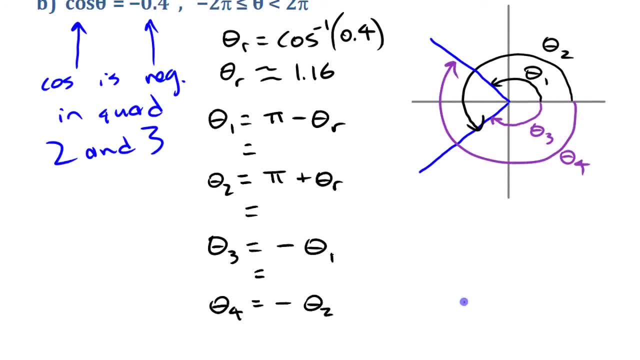 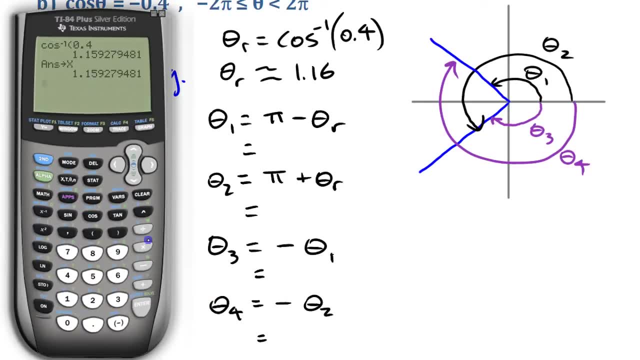 All right, So we'll have our various angles there. Once we're done, let's go back to the calculator and find those. So now, since I stored that number, all I need to do is just recall it here: Pi minus X. 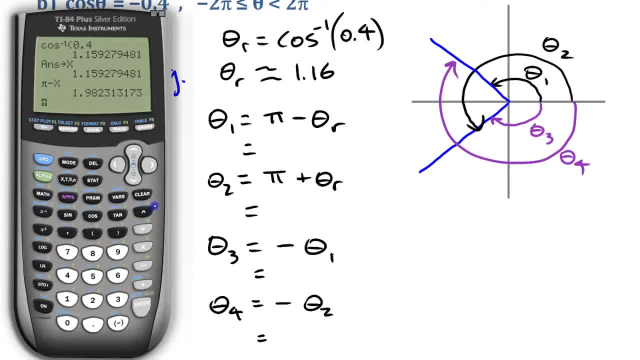 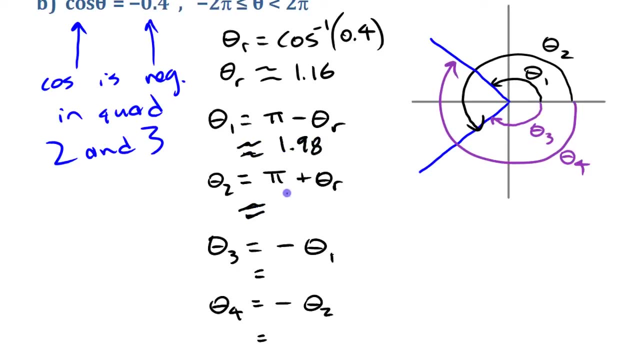 That gives me that value, 1.98.. And then I can do Pi plus X. That gives me that value. So I got 1.98 and 4.30.. Roughly speaking, I should have put a roughly equal to there: 1.98, 4.30.. 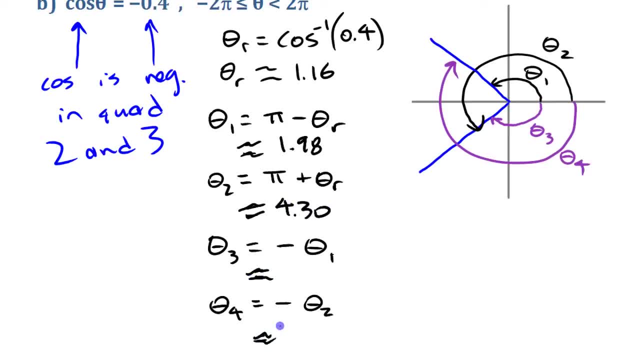 And then the other ones here are just going to be the negative, So negative 1.98 and negative 4.30.. All right, So I want to sum it up over here, And if I want to put them in order, not that it matters. 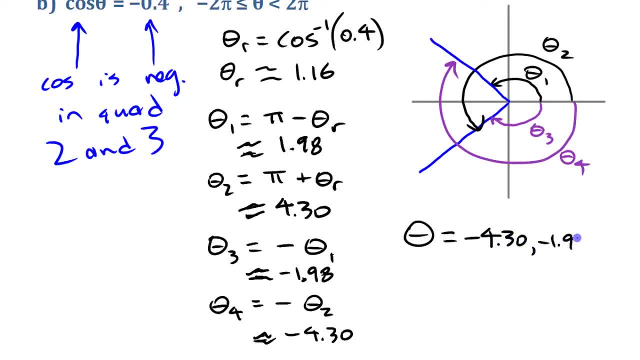 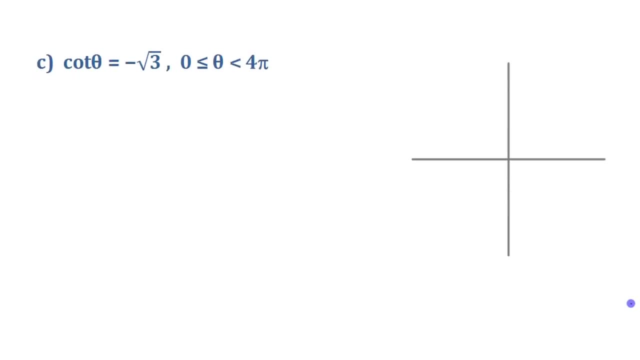 But 4.30, negative 1.98,, 1.98,, 4.30.. There's four angles in that domain that work for that given information. All right, Let's look at one last one here. We're looking here where cotangent is negative, root three: 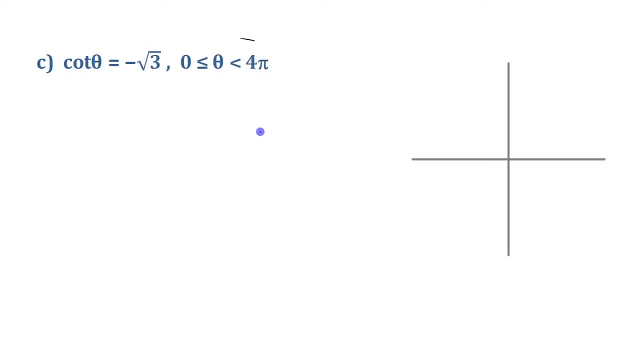 And we have a domain of zero to four Pi. So two full turns in the counterclockwise direction we're looking for Now. we need to think two things here. First of all, we need to think cotangent is negative, The same place as tangent is negative. 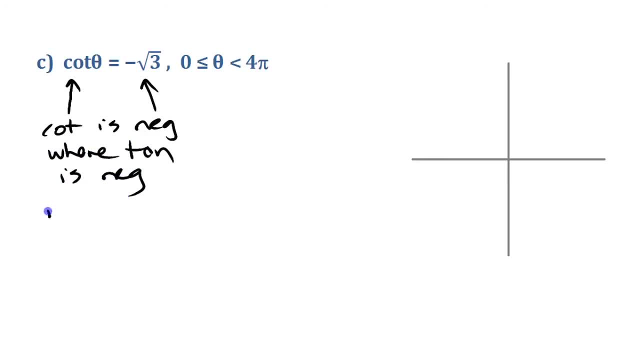 And that is in quadrants two and four. Quadrants two and four we're looking in, So we're more or less going to be looking here and here for some angles. Again, I'm just drawing a line in there for reference, even though it's maybe not drawn accurately. 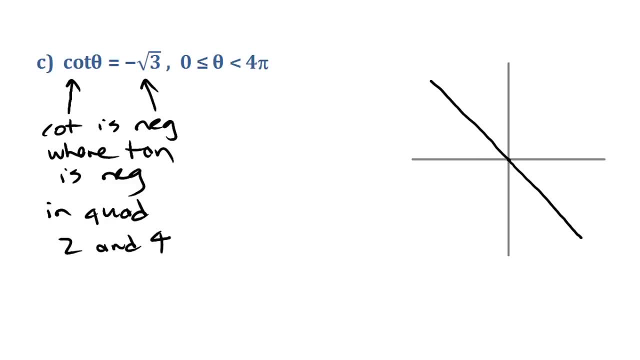 And we're going to be looking for that angle, this angle, and then we can keep going. now, right, I'll do them in a different color here, because we could go all the way around to there, or we could. this is going to get my picture pretty crowded here. 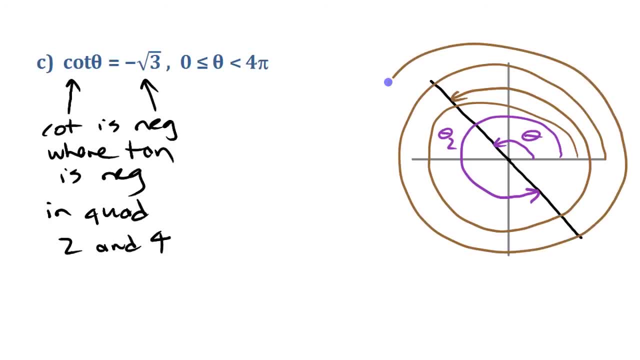 or we could go all the way around like this to there. Now I'm going to erase these, because these are just the previous two angles Plus a full turn. All right, So if I have my first two, Theta one and Theta two, I'm just going to put up here. 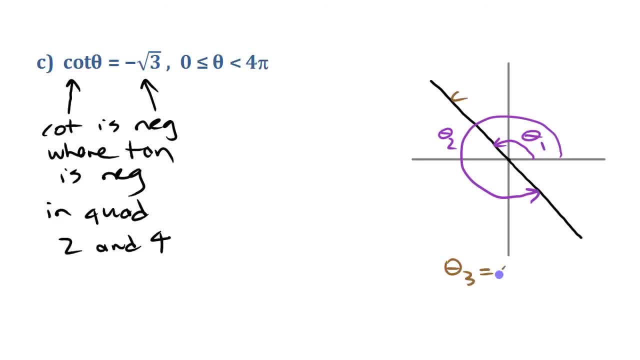 that Theta three is going to be Theta one plus a full turn. All right, If I do that- and plus two pi. and that Theta four is going to be Theta two plus two pi. Or what you might realize is when you're working with tangent, this line, since they're in opposite quadrants, like that. 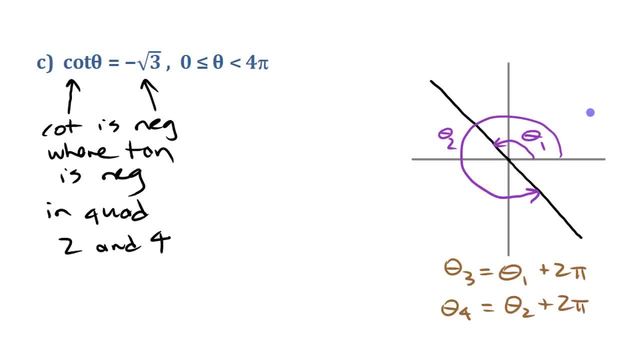 you could actually just take the first one and just keep adding pi to them as you go. All right, We'll get to that in a second here, If we're starting with cotangent, Theta is negative root three. We need to know that. probably it's easier. 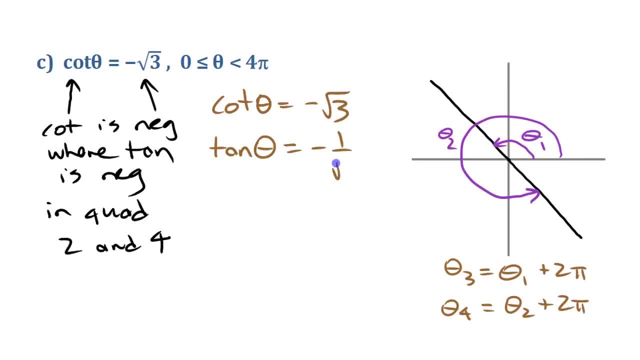 to change it to tangent- is negative. one over root three because it's a reciprocal, And that is a number that you might recognize Because it's one of those values out of a special triangle. So we have this triangle here: one root three and two. 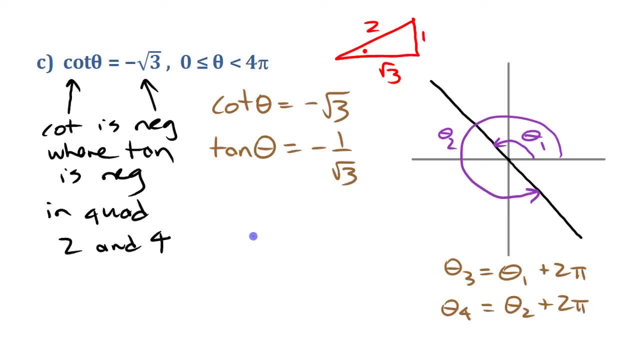 We're looking from this angle Now. we're thinking about how we can get a tangent of one over root three. Well, if this is the opposite and this is the adjacent, then this angle, the smaller angle, 30 degrees or pi over six, is our. 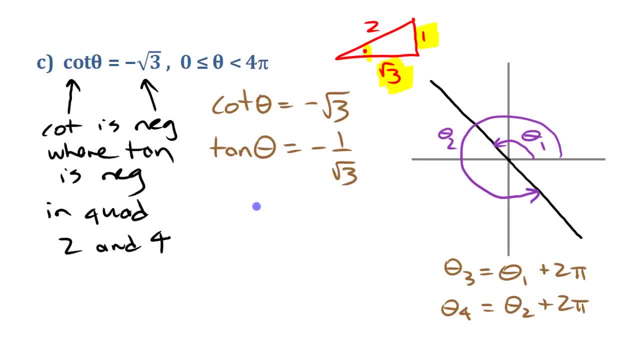 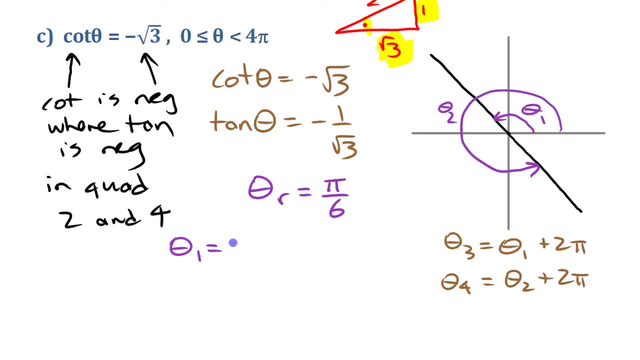 angle is what we're looking for. So I'm going to say Theta reference is pi over six. Now my first angle here. we'll make a list over here. My first angle is going to be pi minus Theta reference. My second angle is going to be two pi minus Theta reference. 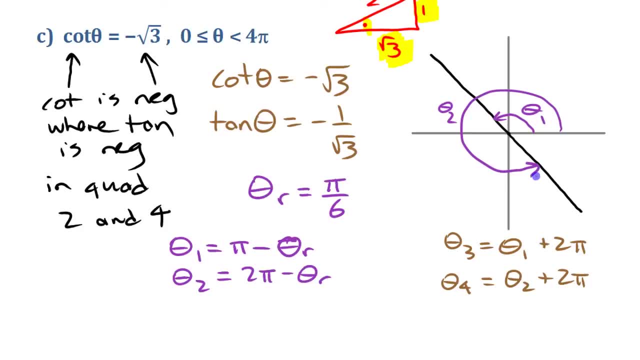 Or again, what we could have done is, instead of saying, Theta two is, you can get Theta two by saying all the way around minus the reference angle, or you can just say it's Theta one plus pi, Right, So you could do it two ways. 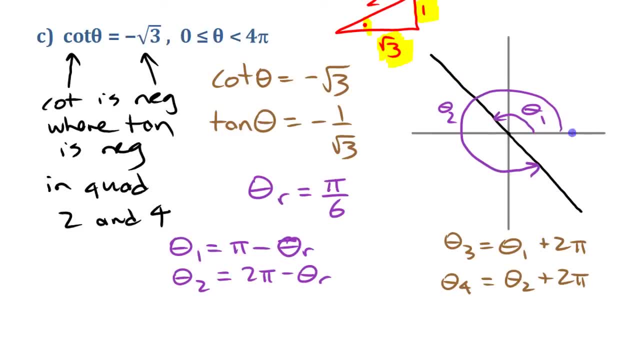 When you're working with tangent or cotangent, you can just keep on adding multiples of pi, because you can say: there's Theta one plus another pi is Theta two plus another pi is Theta three plus another pi is Theta four. All right, Whichever way you do it, you get the same values. 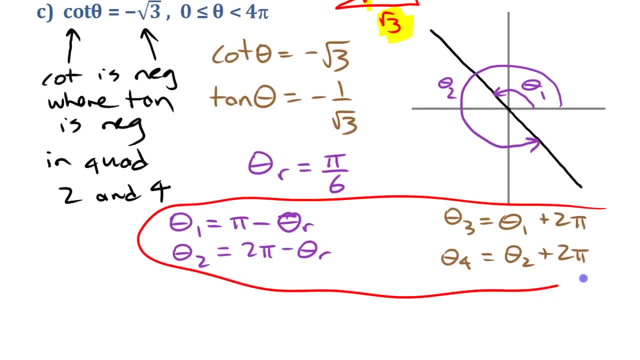 All right, Whichever way you do it, you get the same values. Right, Whichever way you do it, you get the same values. Now I've written out what they all are here. Now I'm just going to write down what they are in a list. Theta is.